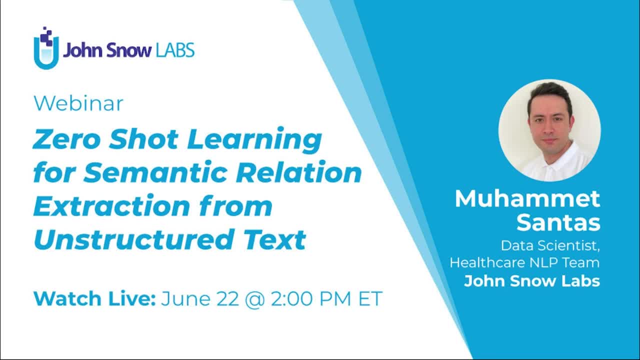 Santas, Data Scientist at John Snow Labs. Today he'll be giving a presentation on Zero Shot Learning for Semantic Relation Extraction from Unstructured Text and how it can apply to and benefit the healthcare industry. So, without further ado, over to Muhammad. 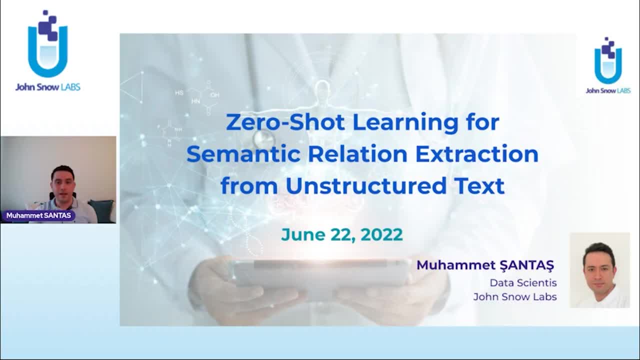 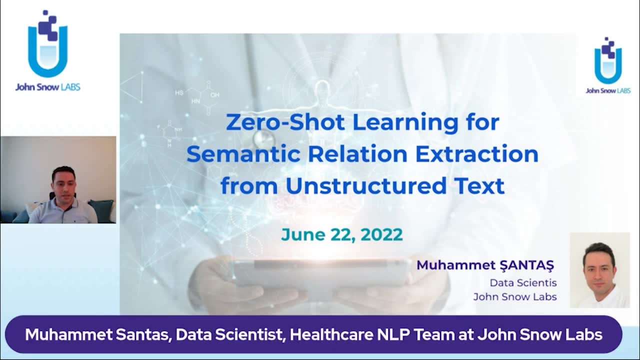 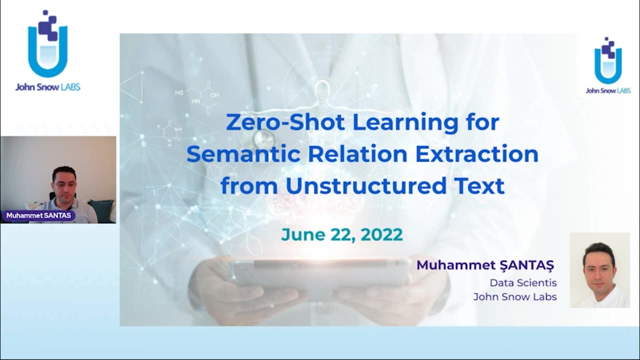 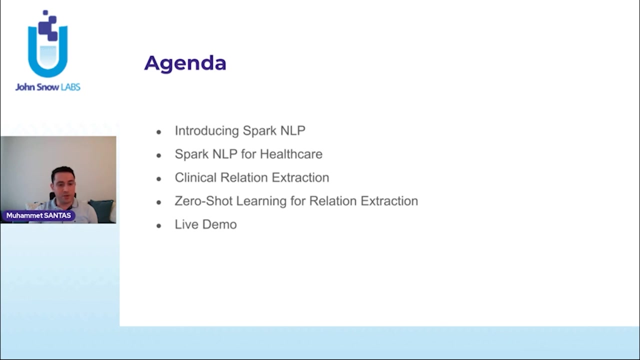 Hello everyone, I'm Muhammad. I'm working as a data scientist in a healthcare team. as Today, we will talk about zero-shot learning for semantic relation extraction from unstructured text. Here is the agenda. We will start with introducing Spark NLP library. 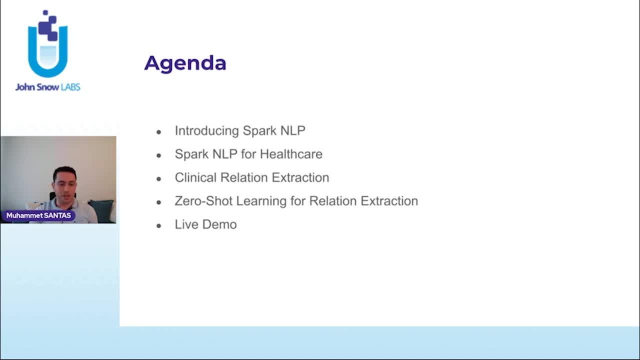 Then we will go through Spark NLP for healthcare and its components. Then I will try to explain how we use clinical relation extraction in Spark NLP. Then we will explain the zero-shot learning for relation extraction in Spark NLP library. At the end of the webinar we will have a live 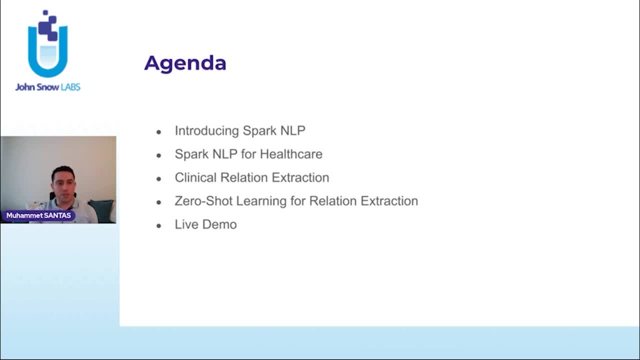 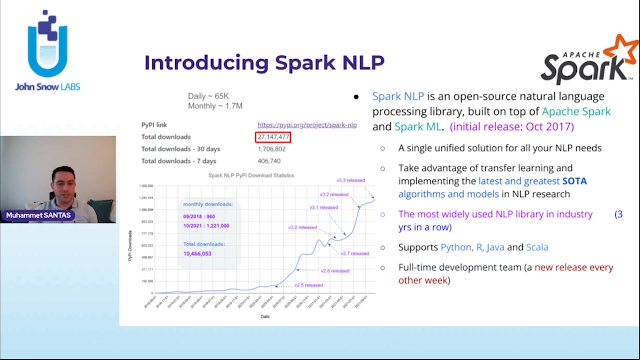 demo session that I will try to show you how we use zero-shot learning in clinical relation extraction in our library. Spark NLP is an open source library which was released in 2017.. The goal was to create an NLP library that would require no other dependencies other than Spark itself. Also, it should work on clusters, since 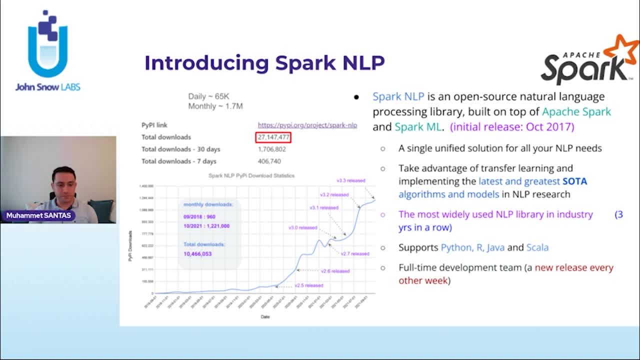 no other libraries could work on Spark clusters. We also wanted to take the advantage of transfer learning and implementing the latest state-of-the-art algorithms and models in NLP. Today we have daily 65k downloads and also 1.7 million downloads in monthly. 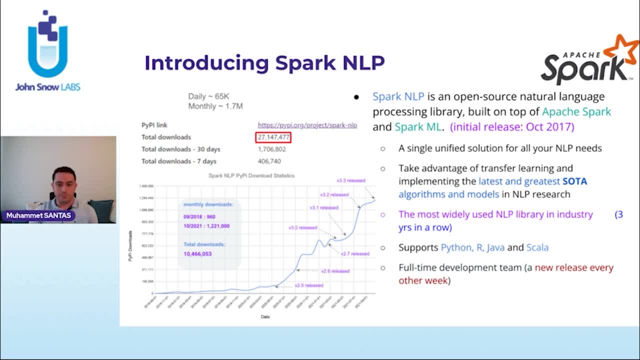 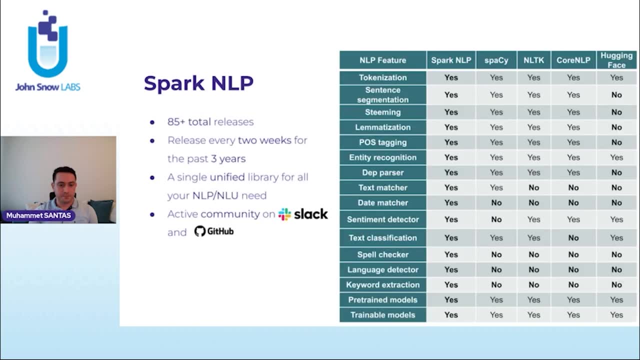 Totally, we hit 27 million downloads so far. Spark NLP supports Python, R, Java and Scala languages. We keep Spark NLP up-to-date and upgraded in every two weeks with new releases. So far we have more than 85 total releases. 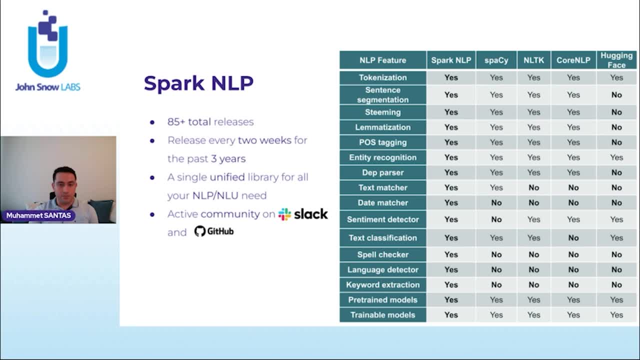 The goal is to create a unified library for all NLP and NLU tasks. You can see some of the features that we have and the other NLP libraries don't Like: date matcher, spell checker, language detector, keyword extraction. Also, we have a dedicated library where you can get all the things you need to know about Spark. NLP and other NLP tasks. You can find this content at the end of our webinar and also our free webinar. In order to use Spark NLP for all your NLP tasks, we have added a link in the description of this video. 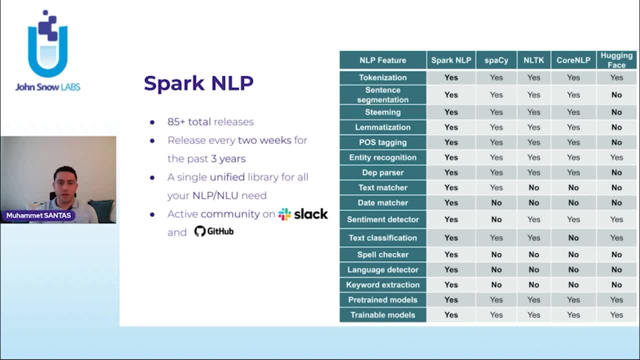 If you would like to add something to your NLP webinar, feel free to reach out to us. If you'd like to add something to your NLP webinar, feel free to contact us. Also, we have an active community on Slack and github. You can ask any questions about Spark NLP on our Slack channels. then you will get a pre-reply. 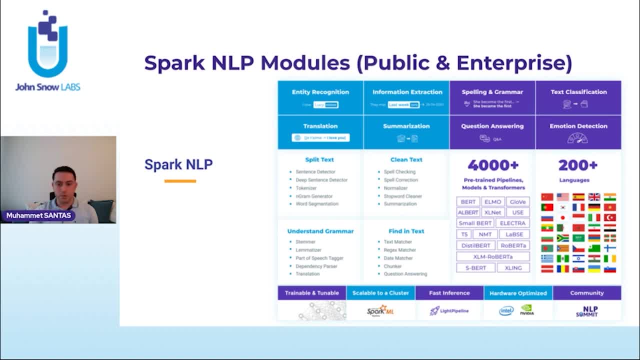 We have public and enterprise versions. You can work for all your NLP tasks, like NER information extraction, text classification, question answering or summarization, by using only Spark NLP. Also, we support more than 200 languages by using the same NER architecture. We have more than 4,000 pre-trained pipelines and models which are trained for different purposes by using different kinds of embeddings like Glow, BERT or Albert. 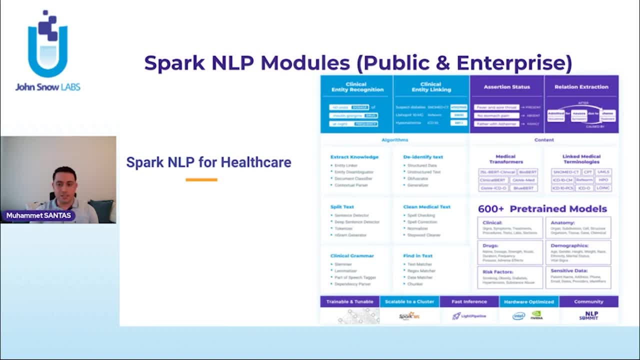 Spark NLP for healthcare is our main focus. We have a licensed library which is special for healthcare tasks And we have also another library- another licensed library that was named as Spark OCR, for processing PDFs, DICOM images or clinical images to get the information inside. But we will not cover it today. 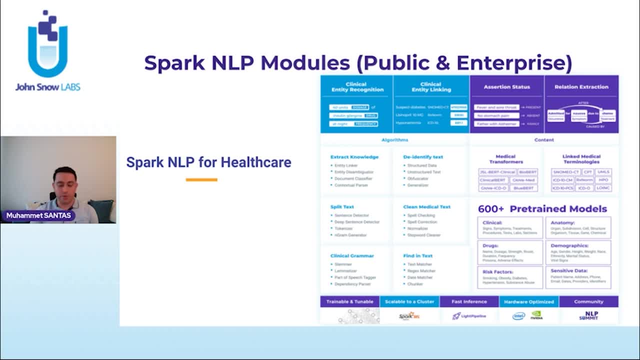 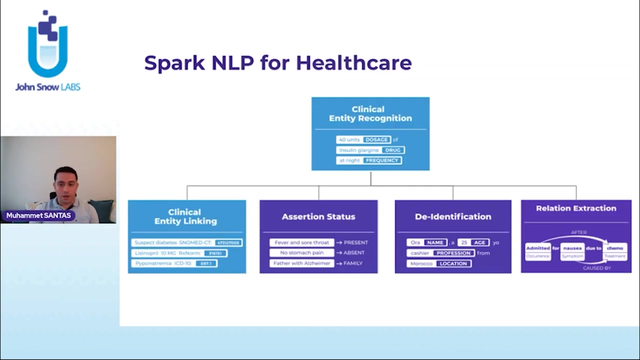 In healthcare module we have more than 600 pre-trained pipelines and models that are trained for different tasks in healthcare, like entity recognition, entity linking assertion, status or relation, extraction, de-identification, chunk mapping and more. Clinical entity recognition is the most important part in 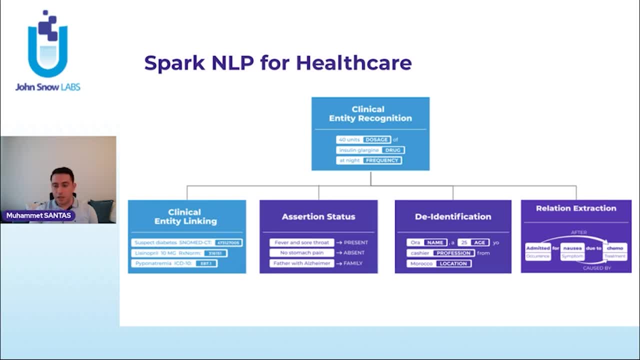 clinicalantenity recognition And the most important stage in health, AAAAAaaAaaaAAAAAAAAAAAT el. Everything is built upon clinical entity recognition. recognition: we have to more than 100 deeply clinical entity models that are triṩing n different kind of clinical 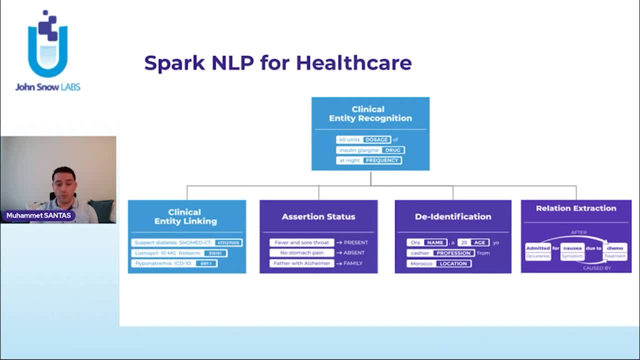 datasets like N2B2challenge dataset or NBCI and onto PodMet out that we live on datasets After getting meaningful chunks. you can use these entities for different kinds of tasks, Like if you get the disease entities or problem entities, you can assign their ICD-10 codes or you can find the additional codes of the drugs. 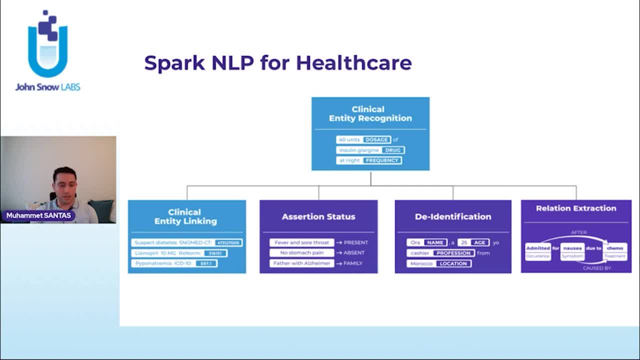 Or if you are working on a clinical test and you need to check if a disease is related with the patient or someone else. You can use assertion status model for this and for the negation status checking the entities. Also, you can use the identification models. 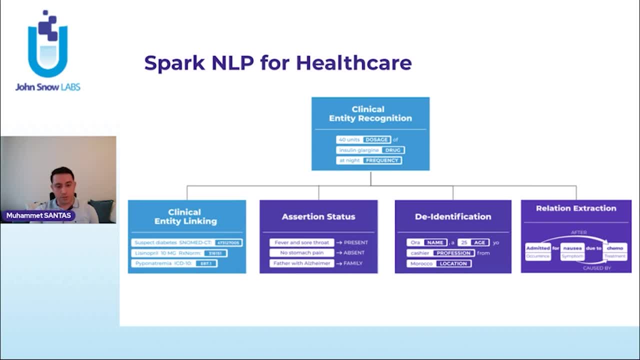 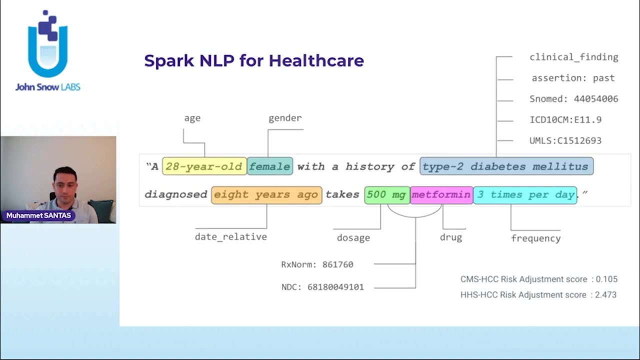 And the identification models, And the identification models And the identification components of our library to identify or obfuscate your sensitive information. Obfuscate means replacing with the fake ones the sensitive information. Maybe you can use these extracted entities and you can find the relations between them. 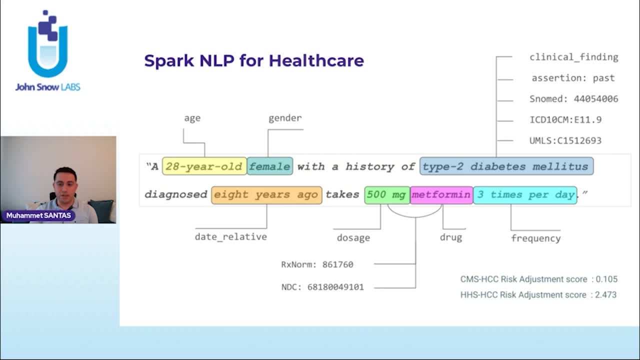 This is the ideal result that you want to achieve at the end of the test. This is the ideal result that you want to achieve at the end of the test By using all these components together. By using all these components together, As you can see here, we can- we are able to detect different kind of entities. 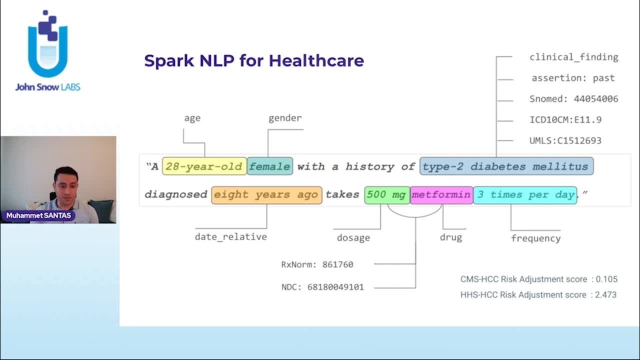 Like age, gender and relative date. Also drug frequency and find their relations. Also find the isolation codes of the drugs. Also find the isolation codes of the drugs And small amount of clinical findings, as you can see here. And also we are able to calculate the risk adjustment scores of patients. 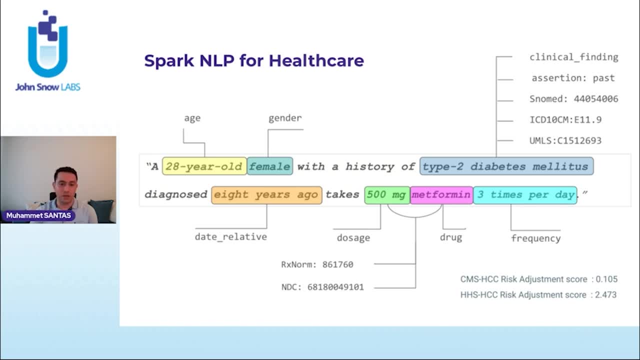 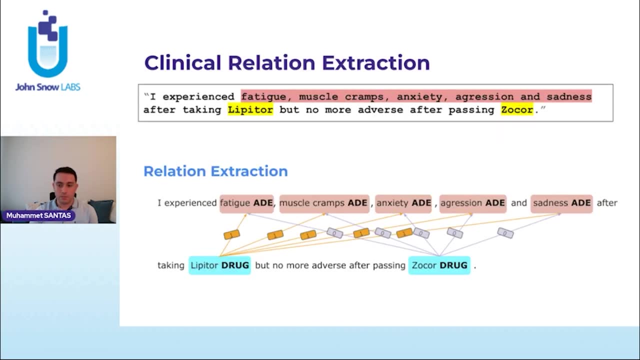 And also we are able to calculate the risk adjustment scores of patients. risk adjustment scores of the patients by using the clinical tests. Clinical relational extraction is one of the most important tasks in healthcare domain. It is the task for predicting the semantic relationships between the detected entities. 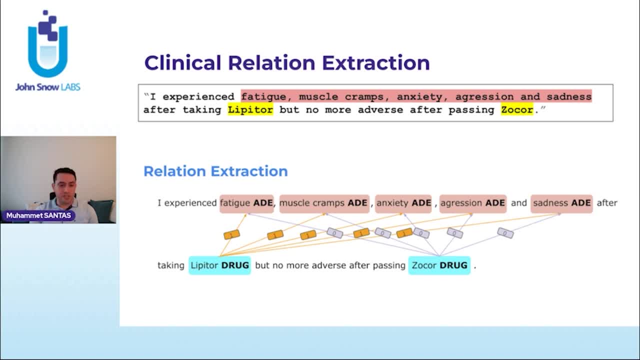 The role of relational extraction in NLP applications are: question answering, summarization, clinical knowledge graph or etc. You can use relational extraction for extracting the many kinds of information from clinical tests. It can be used for detecting the temporal events between the clinical events or you. 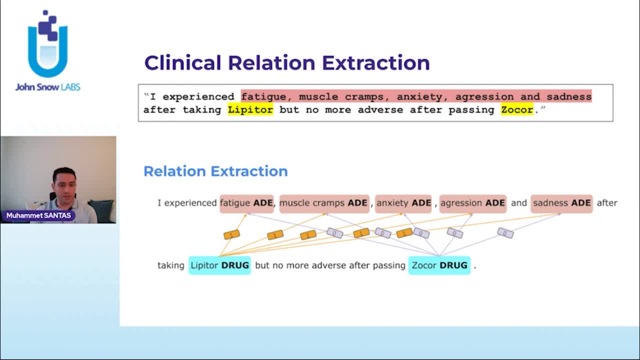 can check the drug-drug interactions or you can find the frequencies between the clinical entities and which frequency is related with which drug or which treatment is used for which problem, If you are working on a task for detecting the adverse drug events as shown in the example. 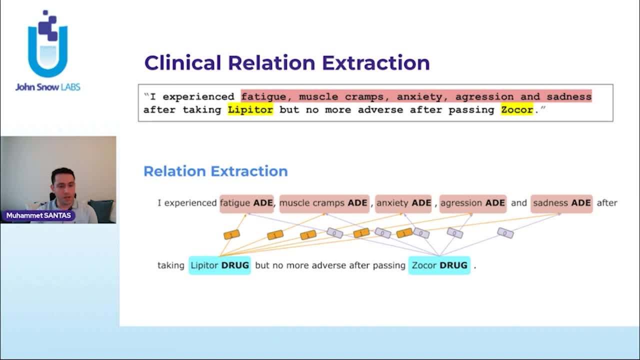 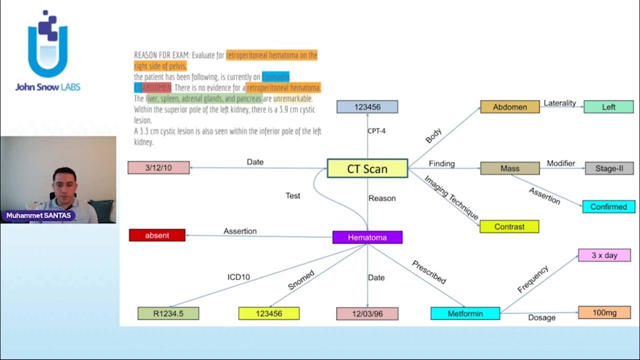 here you may have more than one drug entities in a sentence, and also the ADE entities as well, So you need to check the relations between them, If a drug is Is related with these ADE entities or not. By using all our components, you can get a graph like this: 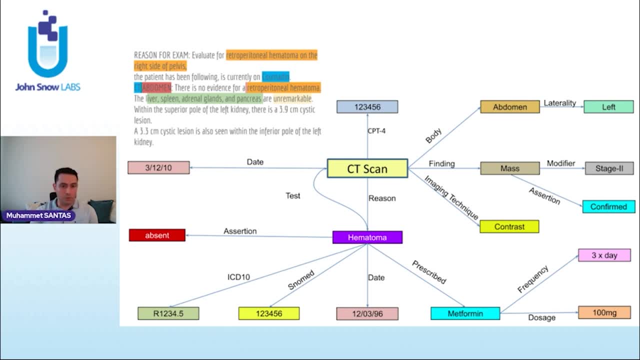 As you can see here. CT scan abdomen. you can see the body, you can see the body parts, body part or findings, or it was labeled as image technique. This is the test for hematoma and the assertion status of hematoma, or ICD-10 code of that. 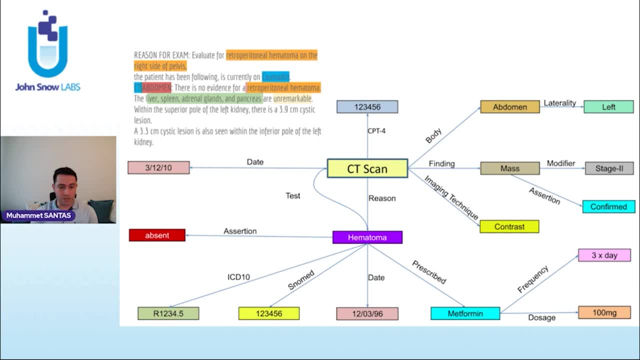 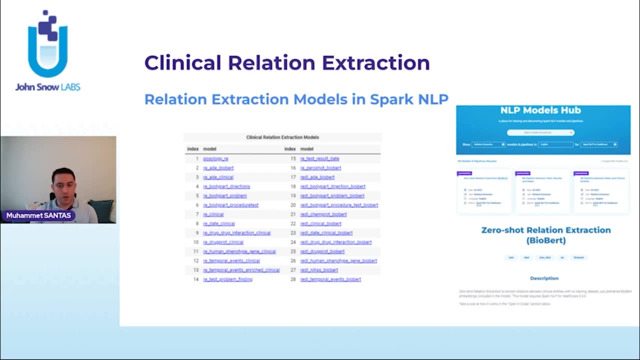 frequencies, prescribed drugs or doses like that. Here are the list of all our relational extraction models we have. We have several kinds of relational extraction models, Trained for different purposes, like ADE and the drug relations or temporal events, or 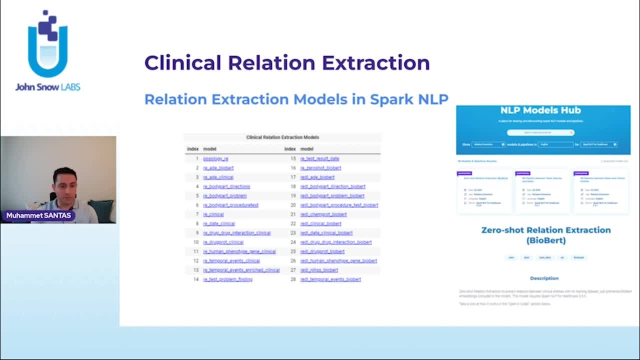 the clinical test dates and the findings. like you can extract the relations between the drug-drug interactions and more. The thing only you need to do is search on our Search for the models on our Models Hub page. then you will see a list of model cards. 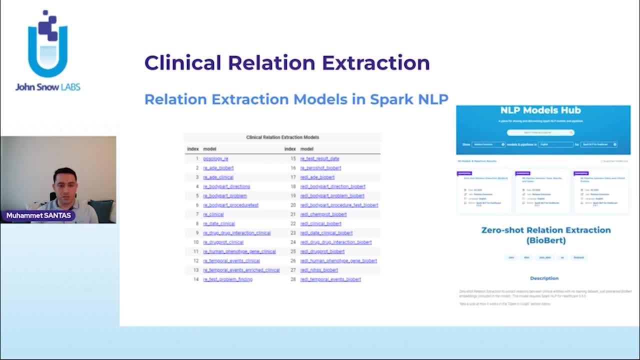 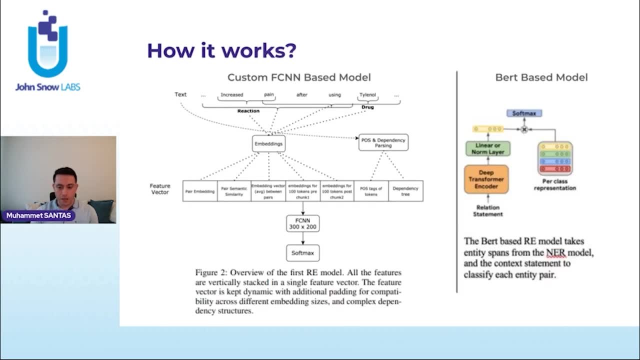 And when you click on them, you will see the descriptions, some sample codes and the other details of these models. We have two different approaches while training our relational extraction models. The first one is Fully connected neural network-based model. The second one is: 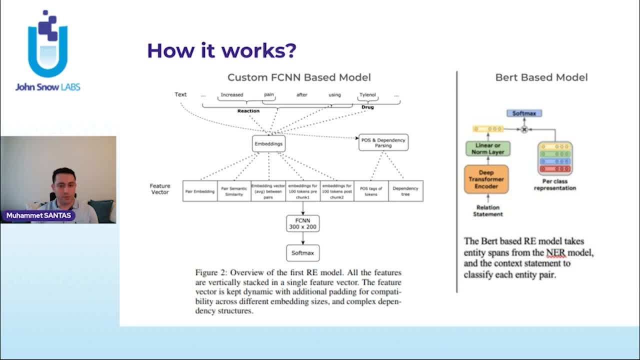 BERT-based model. Why we use two different kind of approach? Because it's for scalability. actually, F-CNN is lighter than BERT, but you may have better results by using a BERT-based model. As you can see in the picture left side, the model checks. 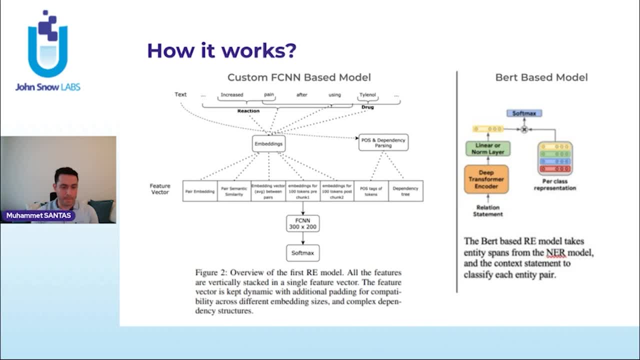 If you want to check The increased pain and the tilling over here, the relation between them, the model checks too many inputs like pair embeddings or embeddings of the tokens from the left side and the 100 tokens from the left side and 100 tokens from the right side, then their 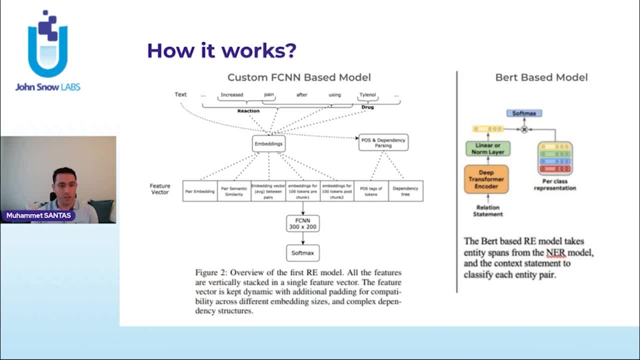 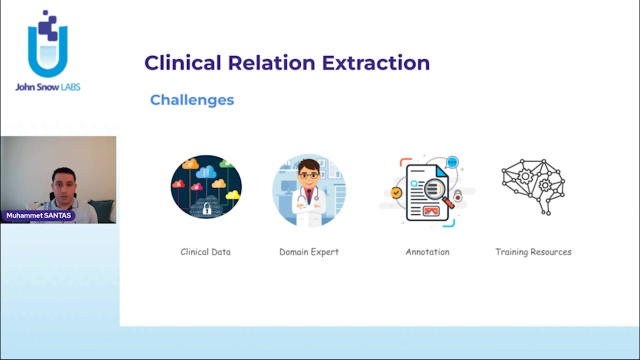 positions and the dependencies between them, Then it returns a result. It returns a result If If these entities are in a relation or not. In the BERT-based one, it works like a sequence classification- end-to-end sequence classification. There are several challenges while training clinical relation models. 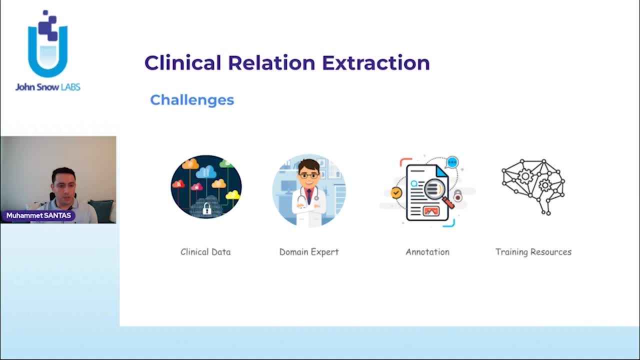 Finding the clinical data is the biggest problem for training a clinical model. actually, Since the clinical data sets contains Some Some sensitive information, like PHI entities, you cannot share them with the third parties. Processing the clinical data sets requires spatial domain information, so you need domain. 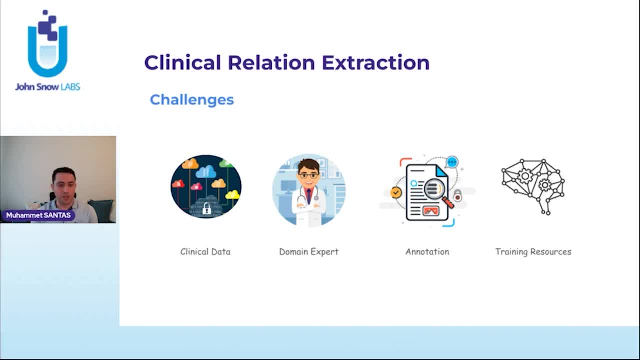 experts to check them. Also, you need an annotation tool for annotating and your domain experts should be trained on annotation. Also, the training resources are the common problem of training, deep learning and machine learning models. If you overcome all of these challenges, then you will get a supervised model. 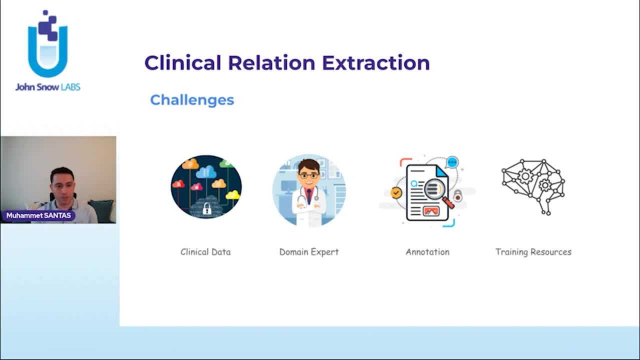 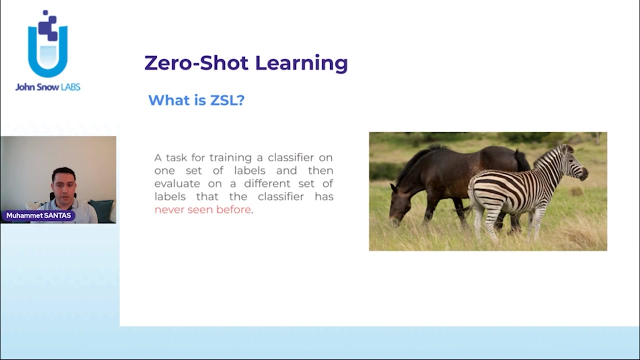 So this means you, You will have a model that was trained, a set of labels, and you cannot use this model for another tasks And you cannot, You cannot, You cannot detect the relations without, You cannot detect the relations if this model doesn't have. 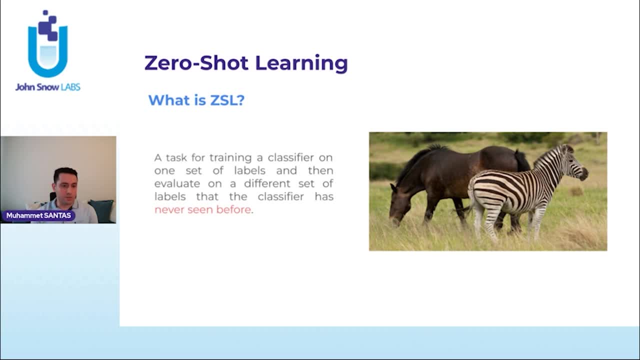 Here is zero-shot learning comes in. What is zero-shot learning? It is a task for training a classifier on one set of labels, then evaluate on a different set of labels that the classifier has not seen before. Let's consider an example: how a child would have no problem recognizing a zebra if he 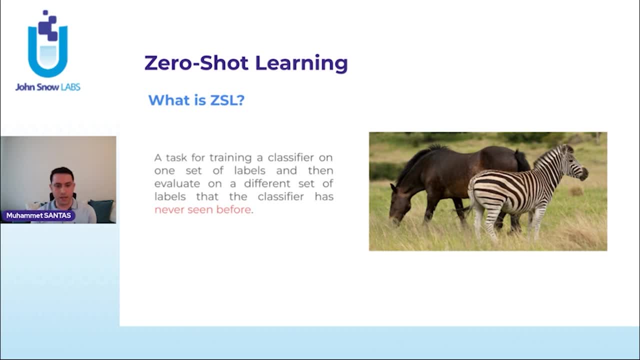 sees a horse before and read somewhere that a zebra looks like horse but it has white and black stripes, He can easily recognize this. This means if you have an adequate information about the object, like appearance, properties or functionalities, You can easily classify or recognize this object. 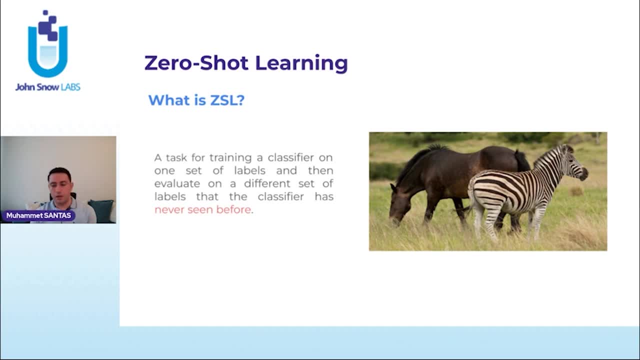 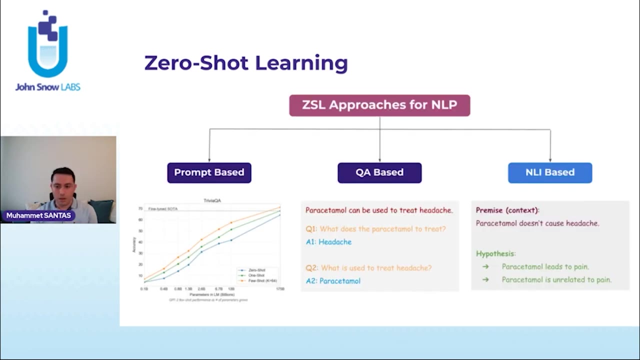 Zero-shot methods basically work by combining the observed and the non-observed categories to some auxiliary information which encodes observable distinguishing properties of the object. Recently, especially in NLP, it's been used much more often. It's been used much more often. 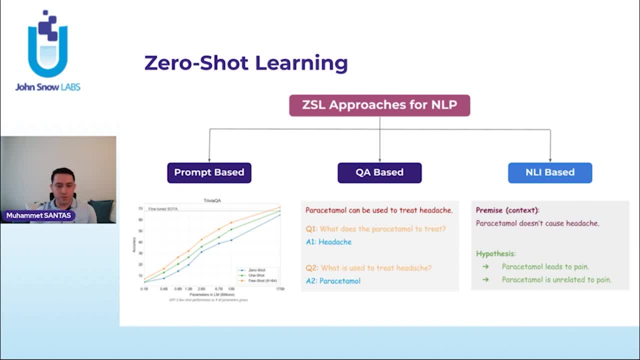 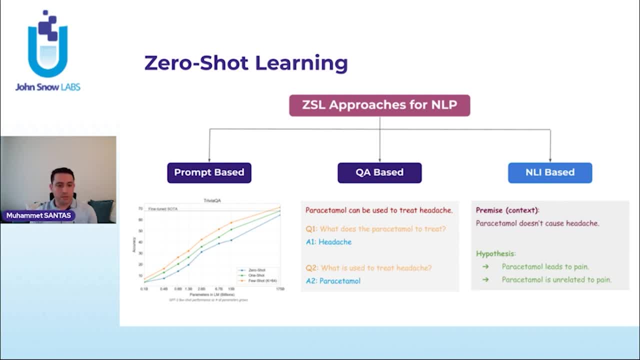 do. There are three common approaches in NLP for zero-shot learning. The first one is prompt-based. As you can see here, the GPT-3 is a good example for this approach. It was trained with 170 examples, 75 billion parameters And the results showed us a zero-shot learning model has a 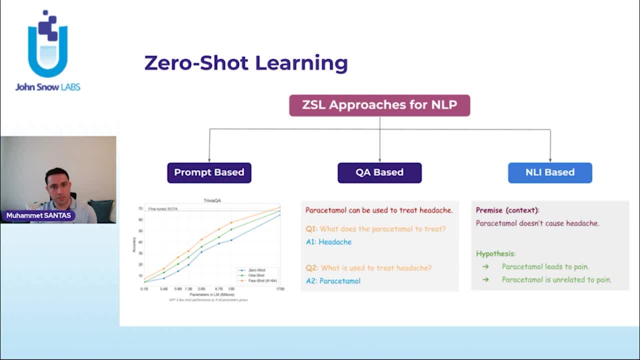 competitively good results with the extremely large language models for downstream tasks And in Q&A based it bases on asking questions and checking the answers for a relation. The NLI-based is the one we used in Spark NLP. Let's take a deeper look in NLI. 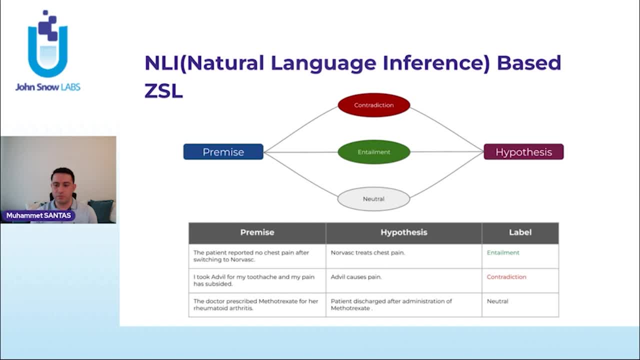 As a quick review, NLI refers to one of the many types of downstream NLP tasks in which a model is asked to identify some relationship between two sentences: premise and hypothesis. NLI datasets are typically modeled via the sequence pair collection. The NLI datasets are typically modeled via the sequence pair collection. 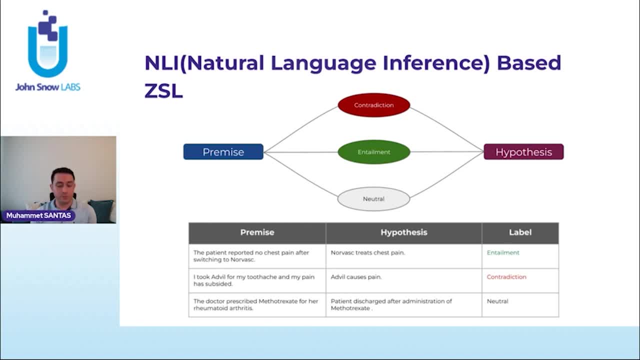 The NLI datasets are typically modeled via the sequence pair collection. The NLI datasets are typically modeled via the sequence pair collection, So we feed both premise and hypothesis into the NLI model. then we get a classification result If the result is entailment, actually if the premise and the hypothesis are compatible. 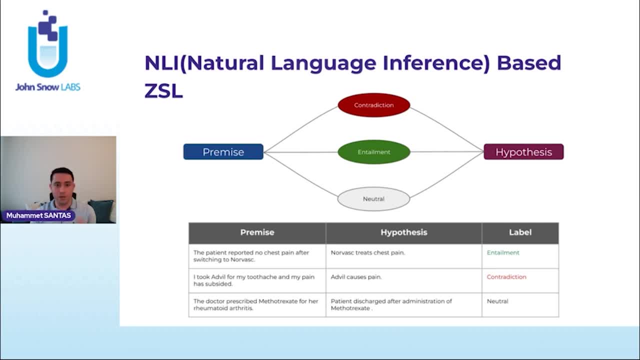 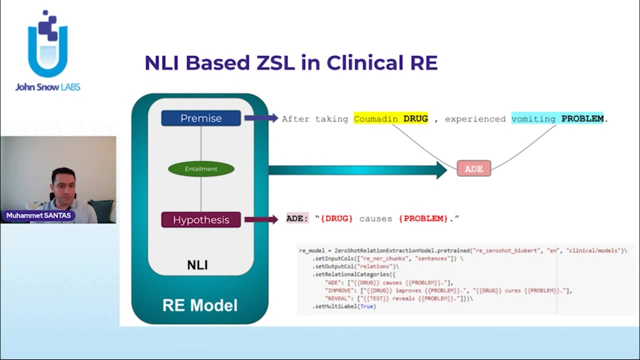 the result will be entailment. If they are incompatible, the label will be contradiction. If they are irrelevant and they will be neutral If they are irrelevant and they will be neutral. If they are irrelevant and the label will be neutral. In Spark NLP, we use NLI-based zero-shot learning. 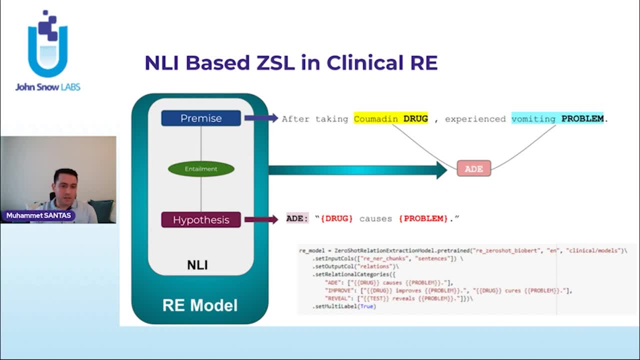 a Phoneme-related expression model. This is how we use it. You can see a clinical test here. This is our premise. After taking Co acquis: highlighted experience wanted. After takingрудin experienced wanted War. summarize: assume that we are working on a task for detecting adverse drug events. 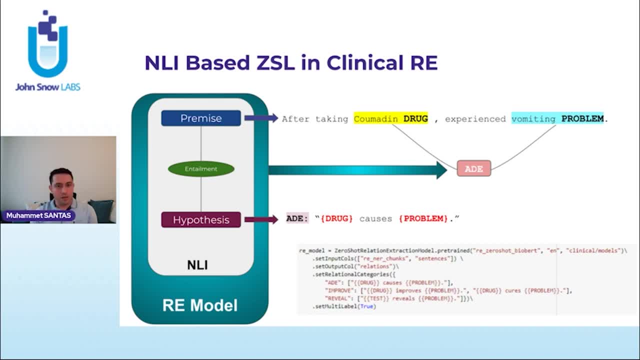 In here. Comodin was labeled as drug and the vomiting was labeled as problem by NER models, So we want to check if they are in an adverse events relation or not. To use our zero-shot learning model, we create a hypothesis. 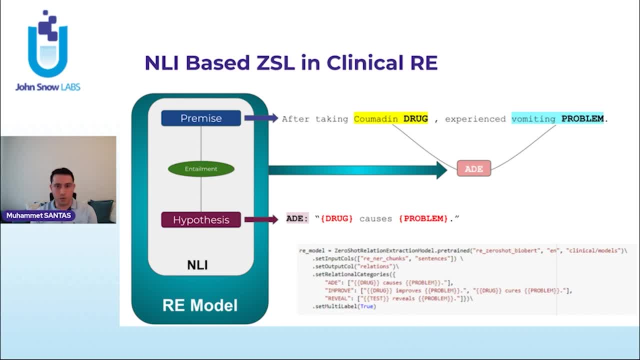 Creating a hypothesis is a tricky point in this model, Because it should be a hypothesis for this relation, For the adverse drug event we created a hypothesis for like a drug-calcis problem. This is meaningful, right. Then we feed these two sequences into NLI model. 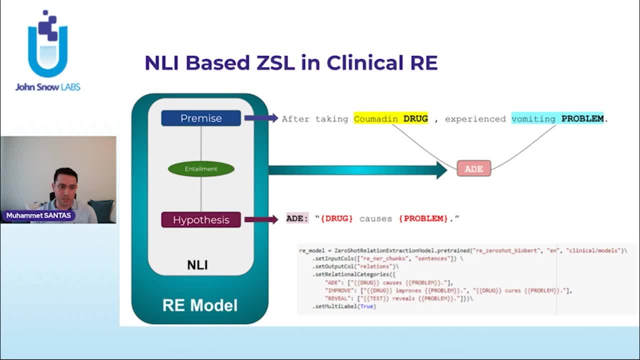 Then the NLI model checks the relationships between these two sequences. And if the result is entailment, the relation is null. So if the result is entailment, the relation is null. So if the result is entailment, the relation is null. 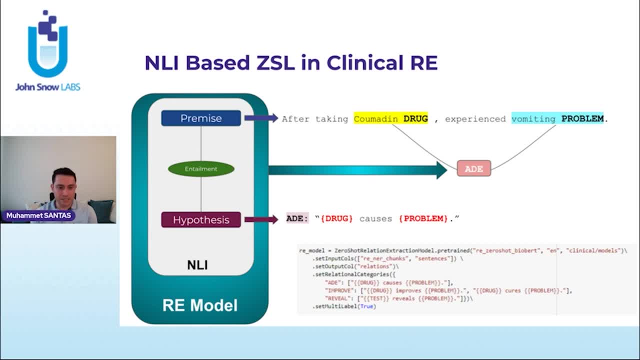 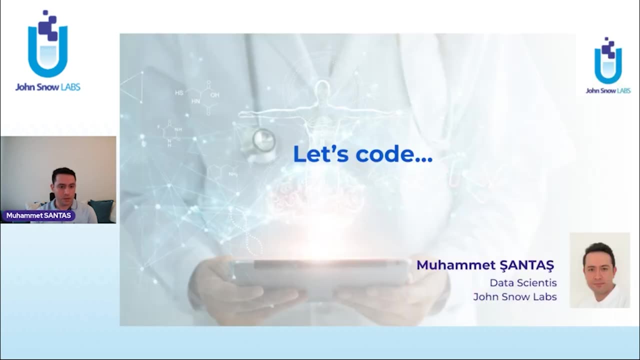 extraction model returns. if these two sequences are in entailment relationship, this means these two entities have an adverse zero interpolation. It is time for presentation. Let's jump into our notebook, then we can. we can. I can show you some examples for how we use. 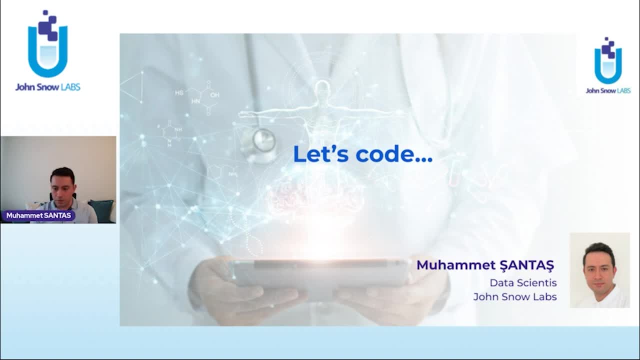 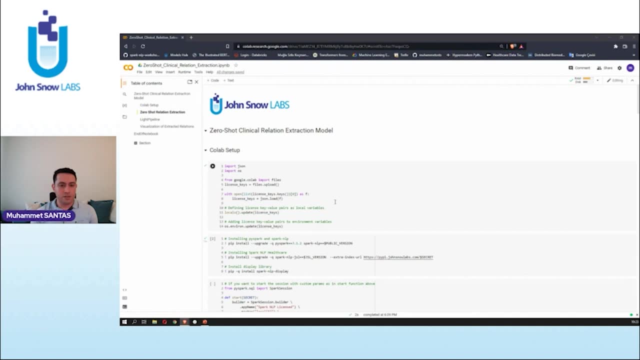 zero-shot learning in Spark NLP. We have a zero-shot clinical relation extraction notebook for you. The first thing you need to do is uploading your license and install the libraries that are necessary for using Spark NLP healthcare model, like PySpark public version of Spark NLP and Spark NLP GSL, which is our. 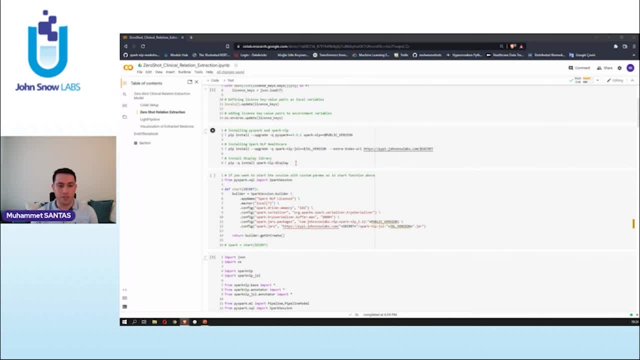 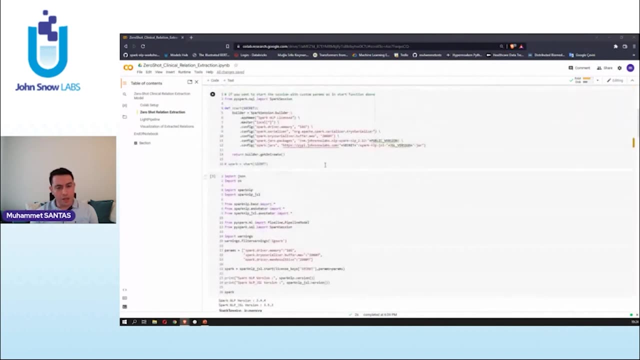 healthcare library and Spark NLP display library, which is for displaying the results. I already downloaded, uploaded my license keys and downloaded these libraries to not to take too much time. You can start your Spark session manually by using Spark builder or just you can use Spark. 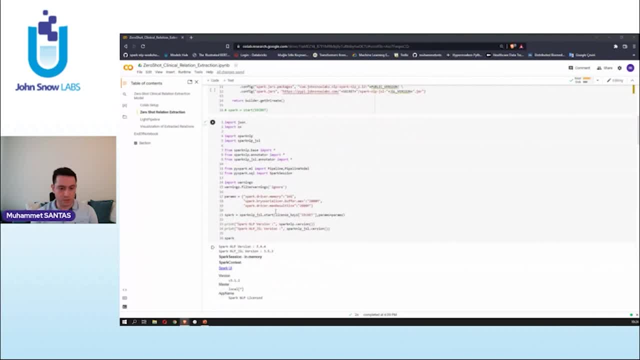 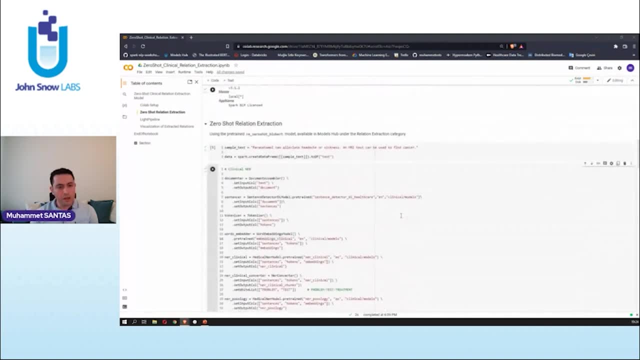 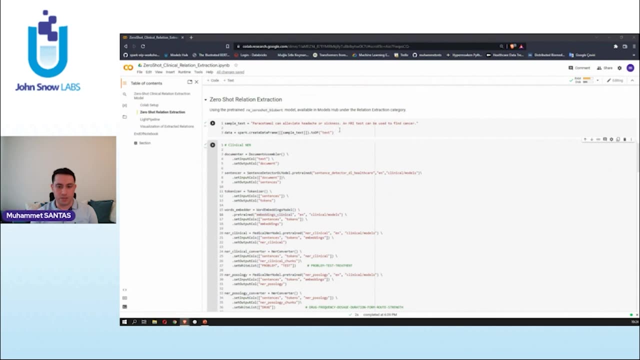 NLP GSL start function. to start your Spark session by providing license key secret. We have a sample text here. Parasitimol can alleviate headache or sickness. An MRI test can be used to find cancer. We create a Spark data frame here by using this sample text. Then we start. 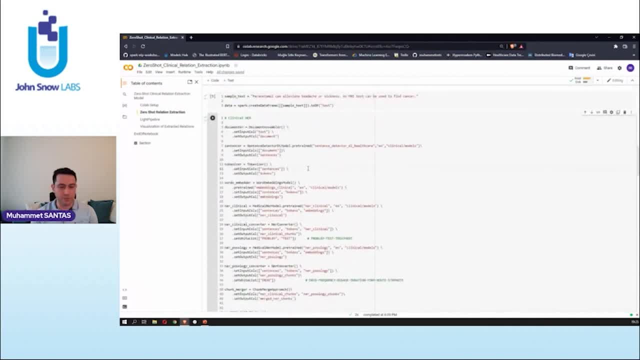 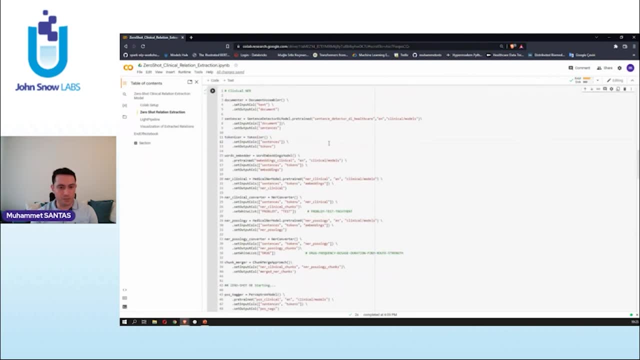 let's take a look at our Spark NLP pipeline. We have a document assembly here. This annotator converts the text model into document type. Then we have sentence. take the healthcare module, which is trained for healthcare tests, and it splits the healthcare text into sentences. Then 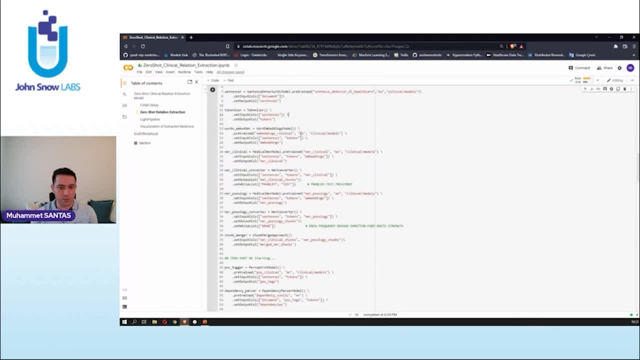 we tokenize our sentences and use our word embeddings model. I used here embedded clinical model, which is used for training these NER models. In this case we have the NER model that we told. actually it requires a pass in this program, which is the stump data structure that we got the kit. 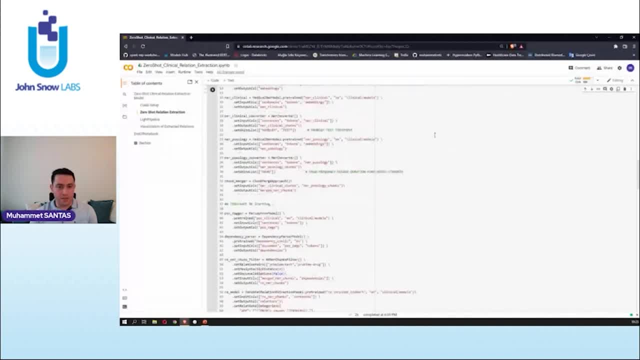 to use for cartography of this program. Also, we have�Multiply 1 NER model of study cases, Certification of NER Williams that we talked about up to 10 years ago, and then those that we have updated on together, as I did here. Yeah, I use clinical NER model which can detect problem test and 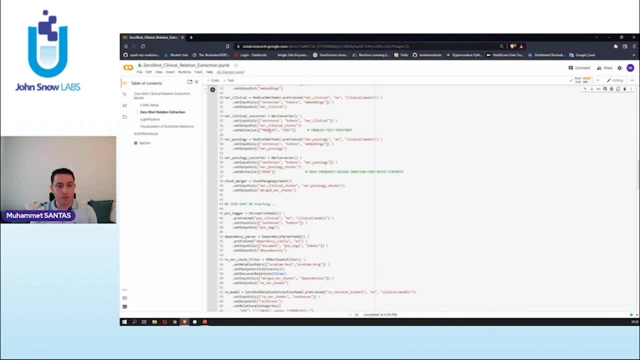 treatment entities in a clinical test, but I use problem and test entities by whitelisting them. Then I wanted to get the drug entities so I used NER pulseology model After that to get a single NER chunk. result: we merge these NER chunks by using our chunk merge. 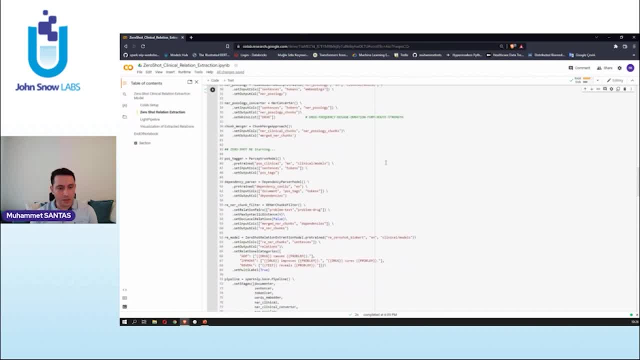 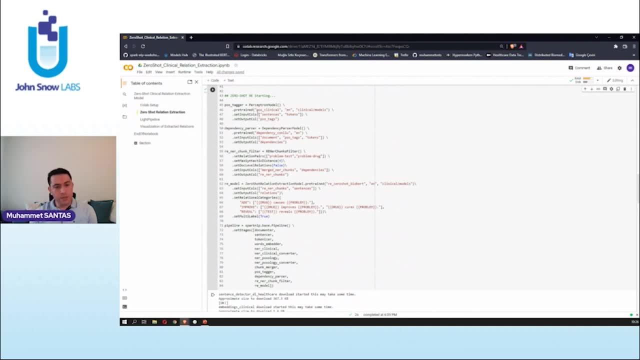 approach annotator and get a single chunk. And here is for our relation extraction model. We use perceptron model to get the positions of the tokens, Then we feed its results into dependency parser model. Then we get the dependencies. After that we filter chunks. 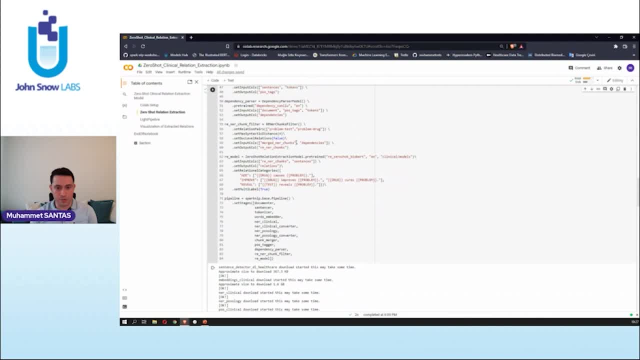 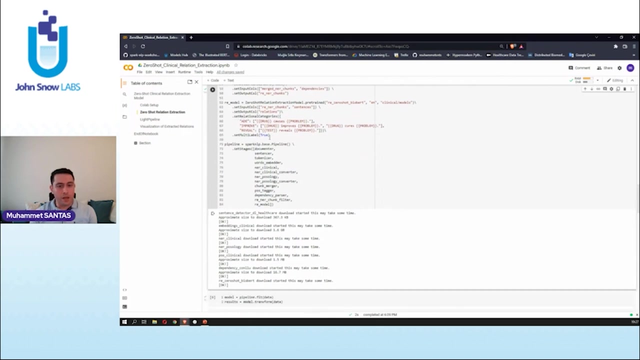 by using dependencies and merge NER chunks. Then we feed its results into, then we feed our zero-shot relation extraction module. that is used for, that is used for zero-shot learning in relation extraction in Spark NLP. We use RE-zero-shot BioWare model here And here. 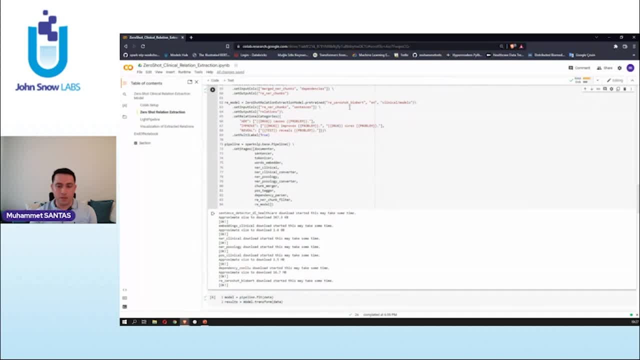 is the most important part. The model has not seen these ADE improve and reveal labels before. So we create hypothesis here You can also create. you can also assign more than one hypothesis, then assign more than one hypothesis, And then you can also assign. 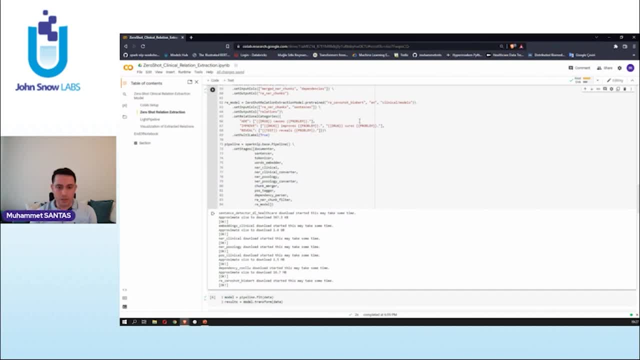 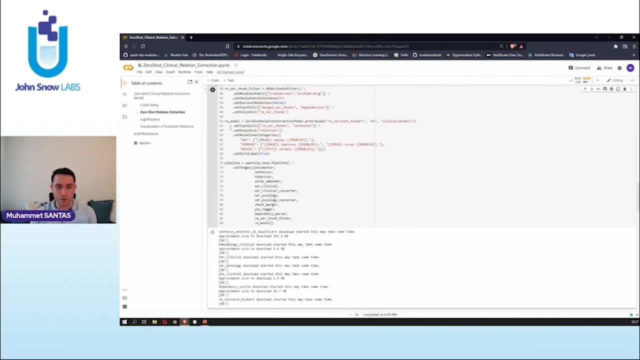 more than one hypothesis, Then assign more than one hypothesis And then you can assign a label for them. The model has not seen these labels before, so we create some rules, hypothesis here. then the model checks the sequences, the premise, our clinical test. 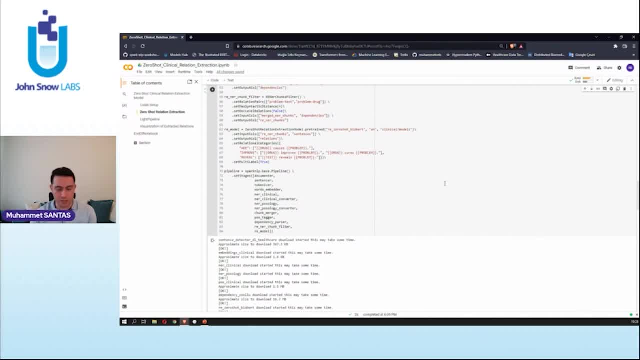 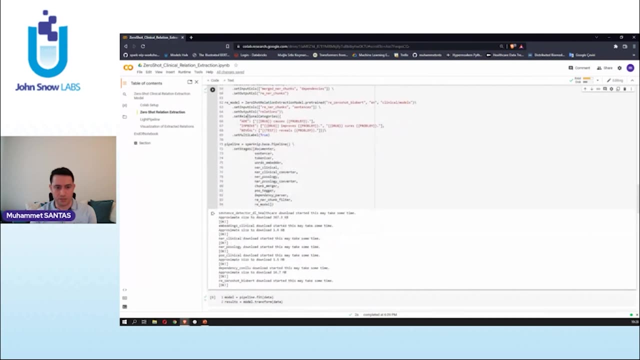 sentence actually and the hypothesis together and the analyte model inside our relation extraction model checks their relationship and if they have an entailment relation, it returns these labels and which hypothesis is in entailment relationship. so the label will be that: 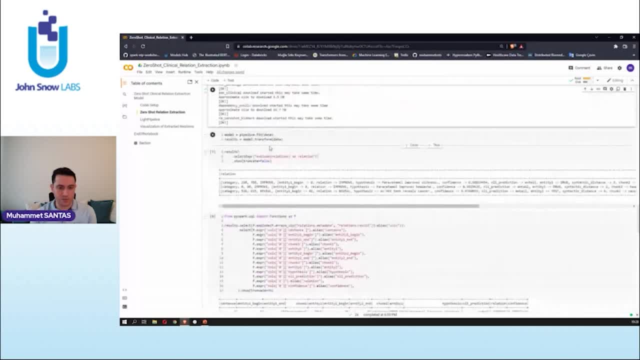 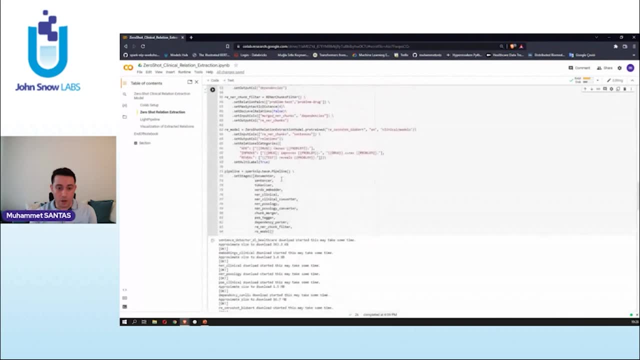 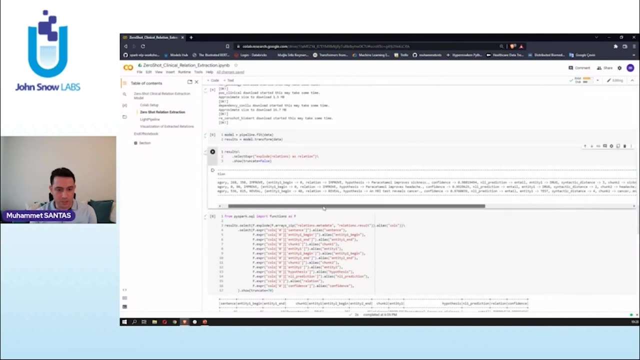 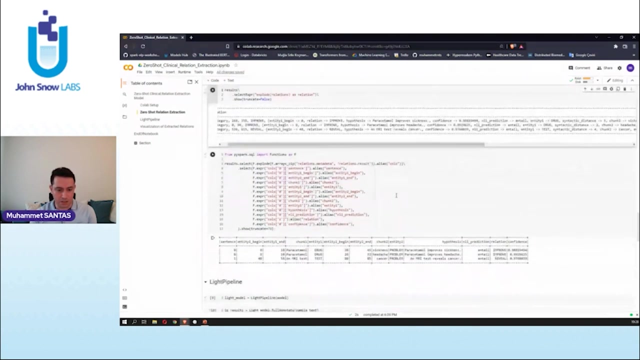 We create a pipeline, then fit the model and transform data by using the model. Here is the results of our output, of our zero-shot relation extraction model. You can see many kind of different, many different kind of information in the metadata like: let's check that in a 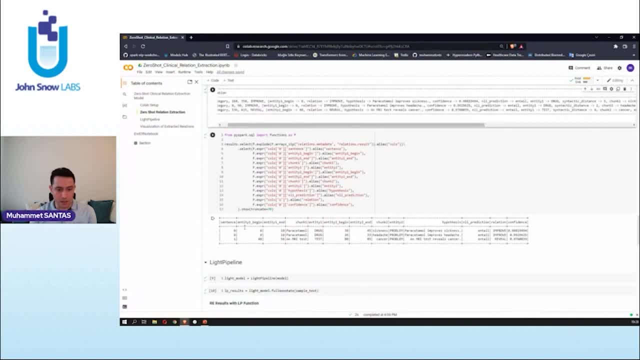 Spark DataFrame you can see that entity 1 and chunk 1, this is chunk 1, paracetamol. it was labeled as drug and here are its beginning and end indices and here is the second chunk, sickness. these are the indices of the second chunk and it's labeled here: problem. 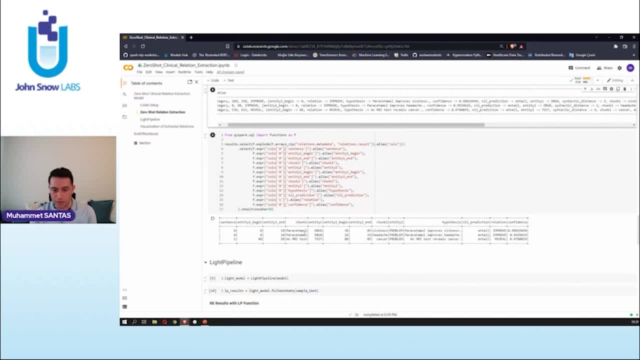 and our hypothesis here. paracetamol improves sickness. The analyte prediction for this hypothesis is entail and the relation label is improve. For the reveal label, our hypothesis is: an MRI test reveals cancer and so the analyte prediction is entail. 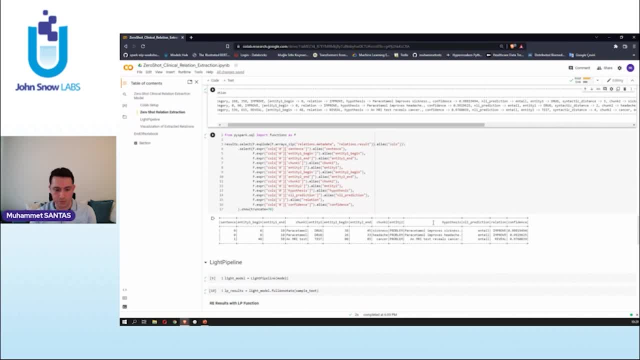 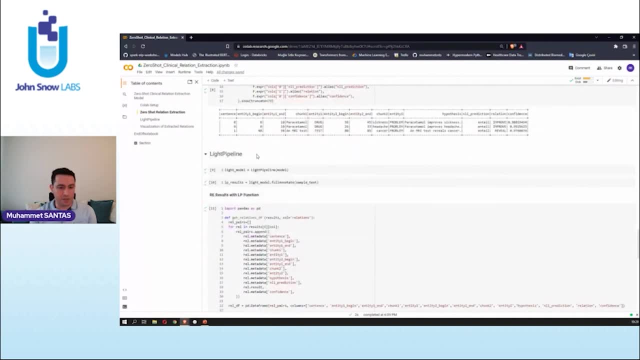 and the label is reveal. You can see also the confidence scores here. Let's use live pipeline. Live pipeline is a special pipeline for Spark NLP. It is equivalent to Spark ML pipeline, but it is meant to get faster results by using smaller amount of data. 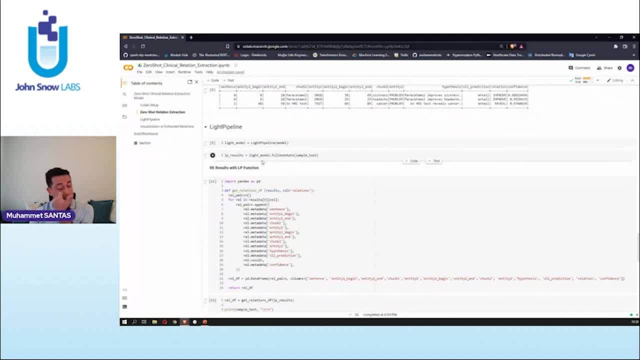 actually, If you have a data lower, smaller than 50k sentences, you can use live pipeline to get a faster result. You can use these results for debugging or checking if you are doing something wrong or you are in a good way for your aim actually. 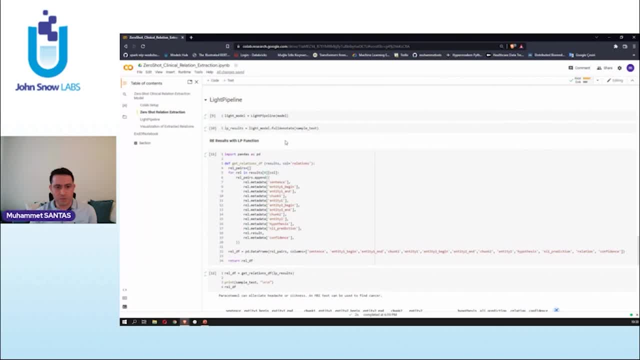 After creating the light model. you can annotate or free annotate. What is the difference between them? The difference between them is: if you free annotate, you get the metadata, and if you annotate, only the results will be returned by the model. So we fully annotate here and define a. 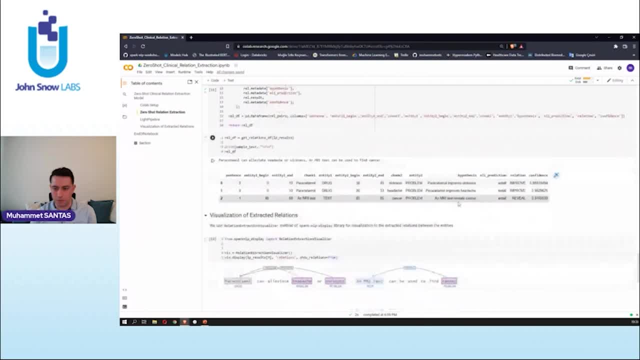 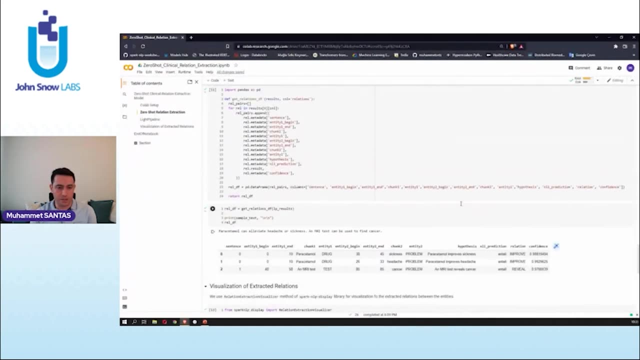 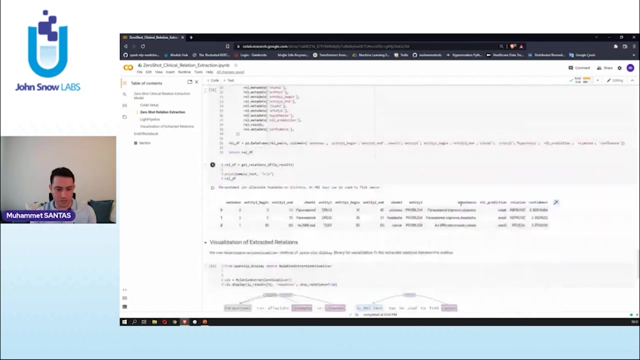 function to see the results in a Pandas data frame. Can you see that This result is the same with the results that we get before, So there's no difference between using the live pipeline and frame according to the results. Let's visualize the results Extracted. 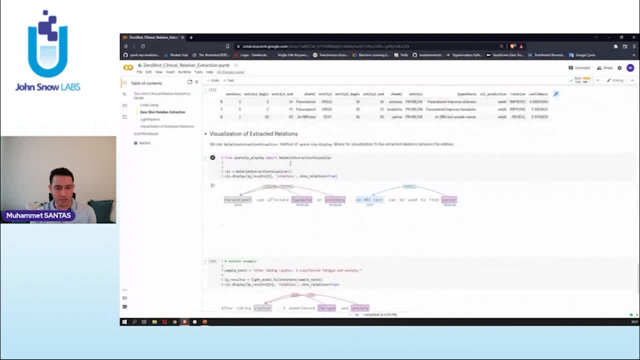 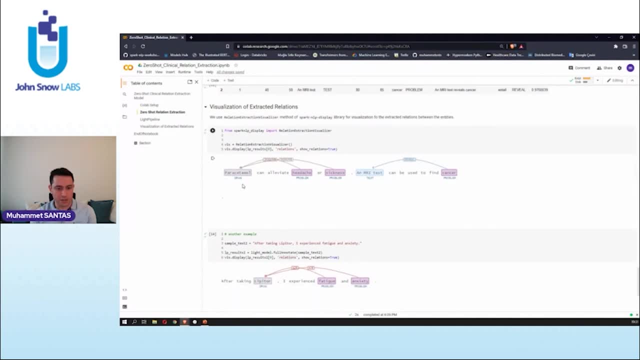 relations. We use SPARC NLP display library and the relation extraction visualizer component here to visualize the relations. Paracetamol can elevate headache or sickness. As you can see here, headache and the sickness were detected as problem and the paracetamol is a drug, So the model says that there. 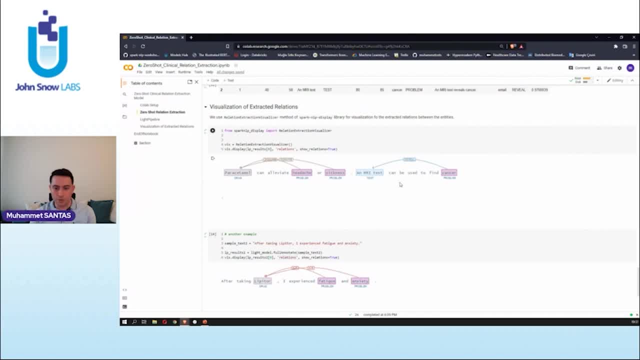 is an improved relation between them, And also an MRI test can be used to find cancer. There is a real relation between these test and problem entities. Let's show another example here. After taking Lipitor, I experienced fatigue and anxiety, As you can remember. 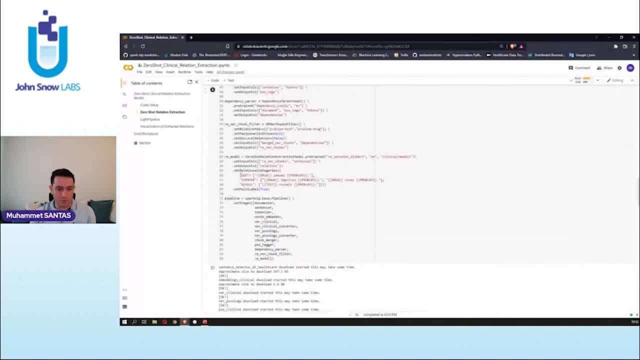 we created a hypothesis for adverse events of drugs. Drug causes problem. This was our hypothesis and here is the result: Lipitor was detected as drug, The fatigue and the anxiety were labeled as problem And the model says that there is an adverse drug-events relation between these two entities. This is the 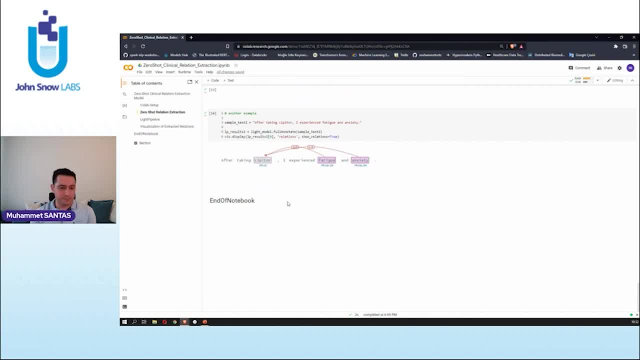 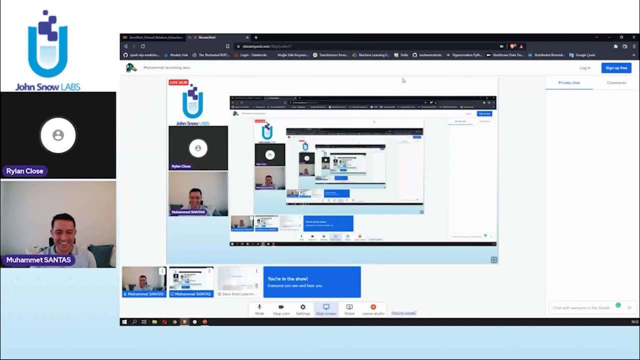 end of my presentation. Thank you for listening. I'm done. Yeah, that was great. I hope it was great. I'm not sure about it. No, it wasn't bad at all. I can end the recording if you're comfortable with that. 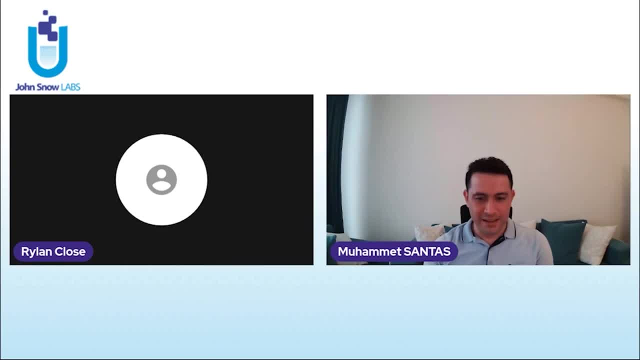